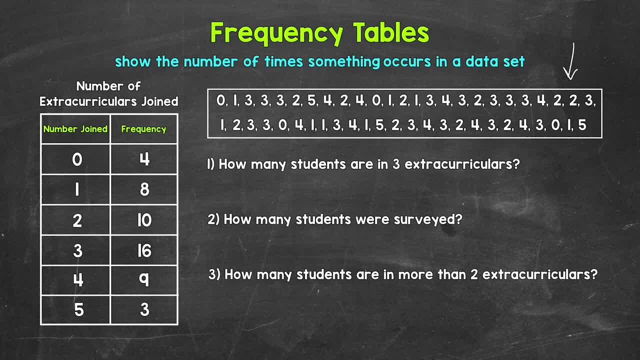 involvement. These are the results. This is the data as it was collected. It has not been organized. This is called raw data. As you can see, this is pretty difficult to interpret and understand, as is. A frequency table will help us organize everything And our 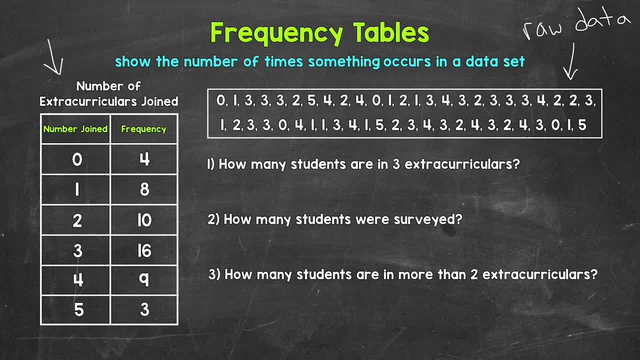 table is right here to the left Now, the left column of the table. so this column right here represents the number of extracurriculars joined, So 0,, 1,, 2,, 3,, 4, and 5.. As far as how I 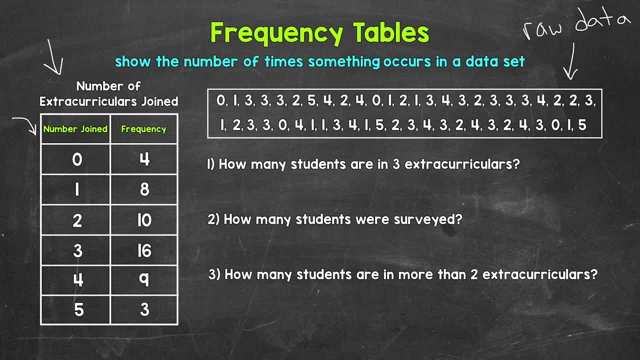 determined which numbers to put there. I just put in the number of extracurriculars that were joined. Now this went from the smallest number in value in the data set- so 0, to the greatest number in value, 5.. Now this is considered ungrouped data because we have individual values in this column. 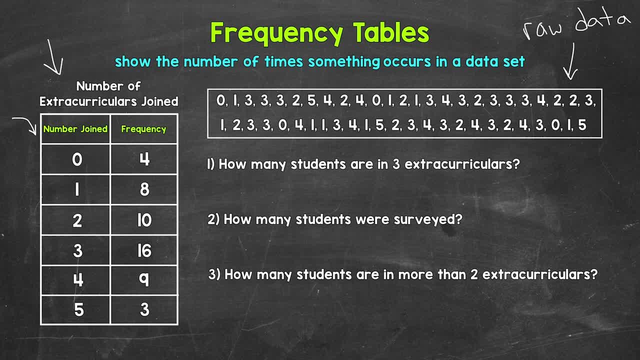 not groups or ranges. You'll see what I mean by groups, grouped data. when we get to that example, You'll see the difference And then on the right side, the right column, right here we have the frequency, the number of times those values show up within the data. So, looking at the 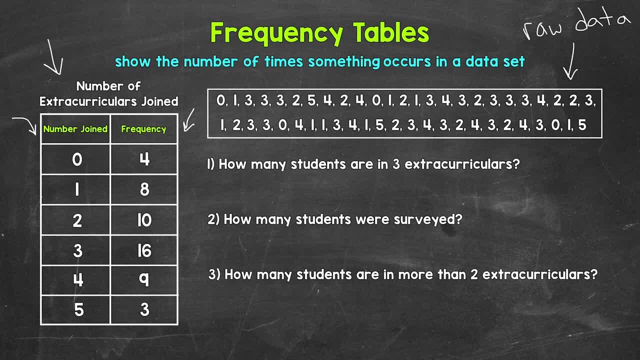 table. let's read this table here. How many students aren't in any extracurricular activities? So 0 extracurriculars. We look right here: Number joined 0. There are 4 students, So 4 students. 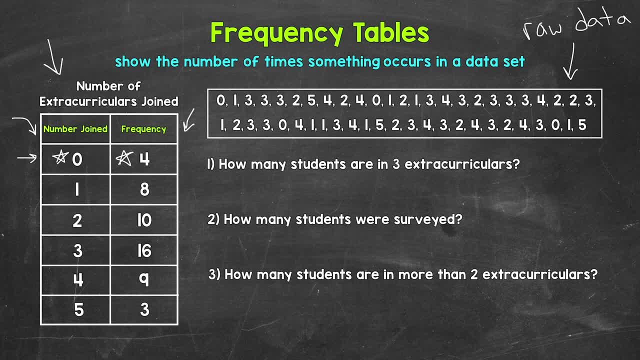 aren't in any extracurriculars. How about 1?? Well, there are 8 students In one extracurricular activity. How about 2?? Well, 10 students. 3?. There are 16 students. 4?. 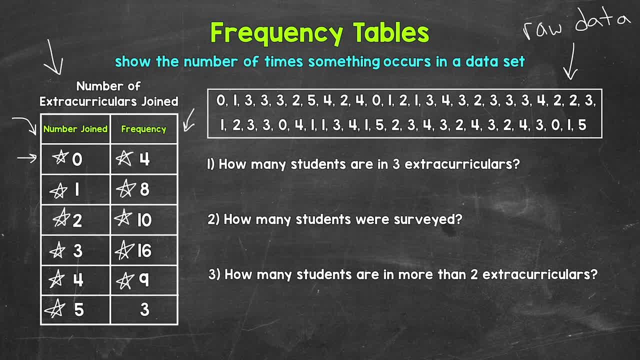 There are 9 students And then 5?? There are 3 students. So you can see that this frequency table really helps organize and present the data in a meaningful and easier to understand way than to look at the raw data. Now let's answer some questions regarding the data, Starting with number 1, where we have 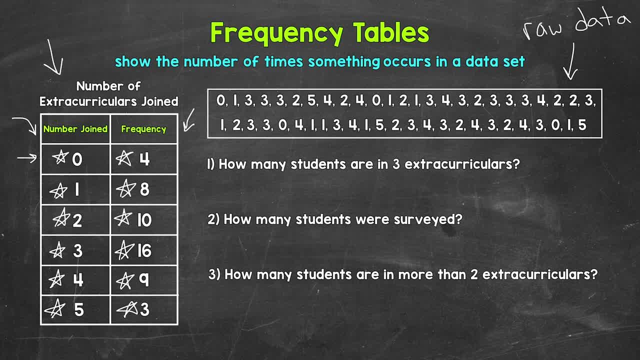 how many students are in 3 extracurriculars? Well, 3 extracurriculars joined, There are 16 students. So 16 students that are in 3 extracurriculars. Let's move on to number 2.. How many students? 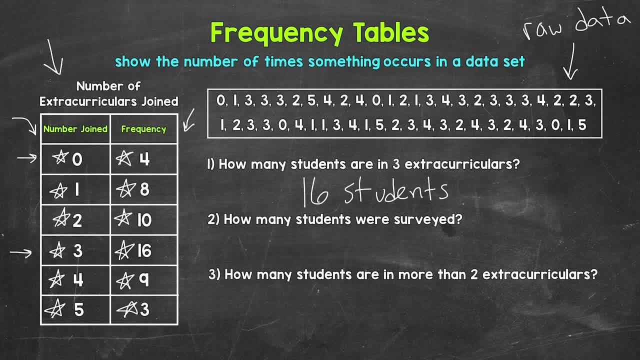 were surveyed. So we need to figure out how many students are in 3 extracurriculars. many total students were surveyed. We do this by looking at the frequency column and adding all of those numbers up. So four students plus eight students plus 10 students plus 16 students plus. 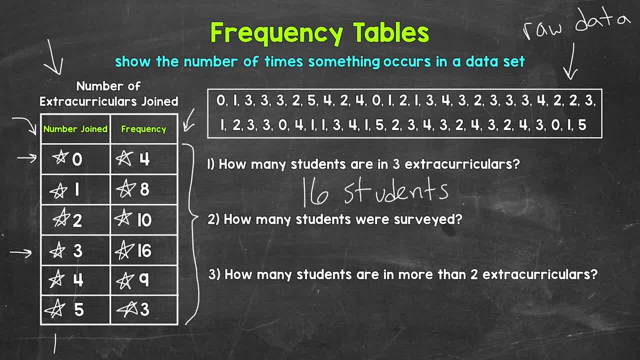 nine students plus three students, So the total is going to equal well, four plus eight is 12, plus 10 is 22, plus 16 is 38, plus nine is 47 plus three is 50. So 50 students were surveyed. 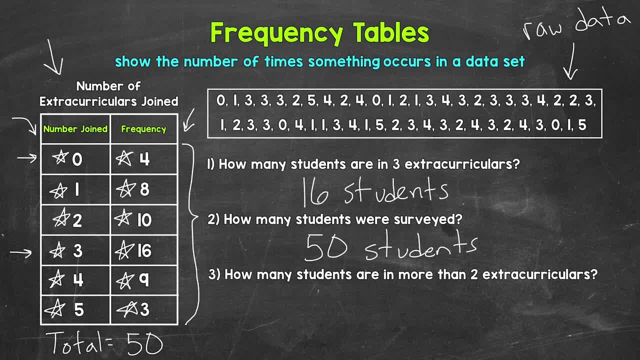 Lastly, let's move on to number three, where we have how many students are in more than two extracurriculars. So two is not included here. We need more than two. So we need to do this by looking at the frequency column and adding all of those numbers up. 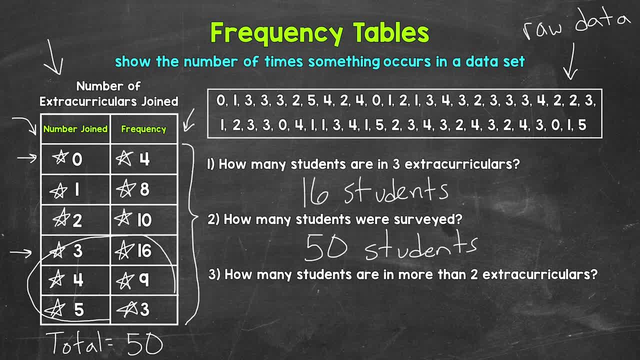 So we need to look at three, four and five. Well, 16 plus nine is 25 plus three is 28.. So 28 students are in more than two extracurriculars. So there is our ungrouped example. Let's move on to our 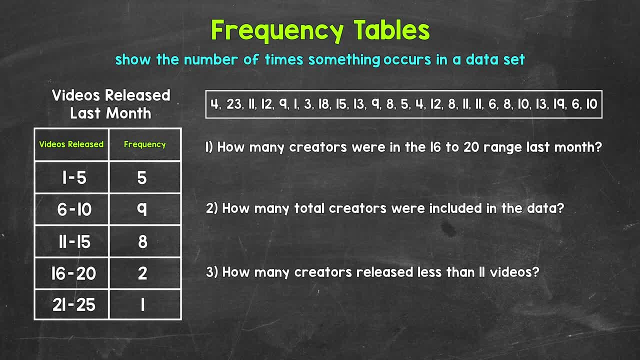 grouped example. Now we will take a look at grouped data, So a grouped frequency table. Let's jump into our example, where we are going to take a look at a frequency table that is displaying this data right here. These numbers represent the number of videos released last. 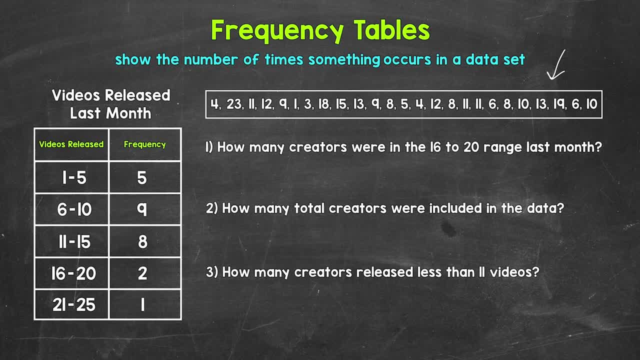 month by a group of content creators, So a certain number of creators were asked about the number of videos they released last month. These are the results. Now, this is raw data. That just means that this is the data as it was collected. It's not organized at all, So you can. 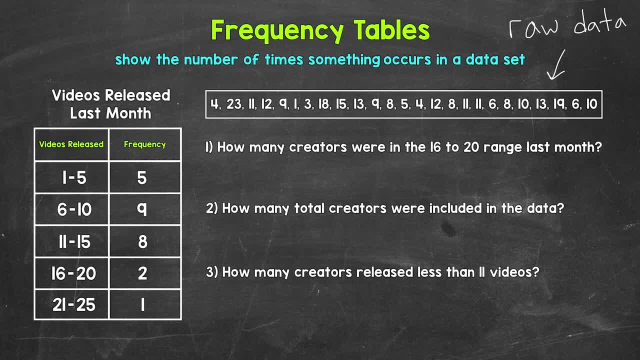 see it's difficult to interpret, as is A frequency table will help us organize everything and our table is right here to the left, Now the left column of the table. so this column going down right here, that's the number of videos released. So this is the number of videos released last month. 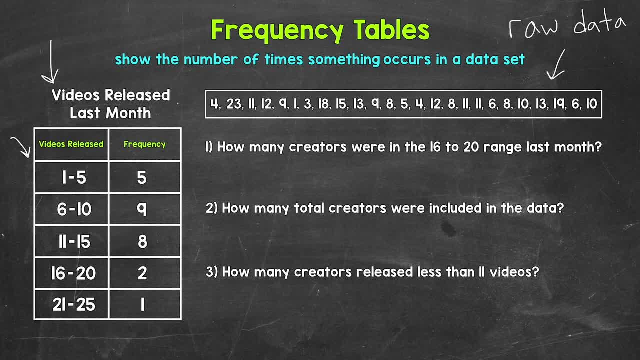 So we have 1 to 5 videos, 6 to 10 videos, 11 to 15 videos, 16 to 20 videos and then 21 to 25 videos. Now these groups are called classes or class intervals. Since we have these classes, these groups, 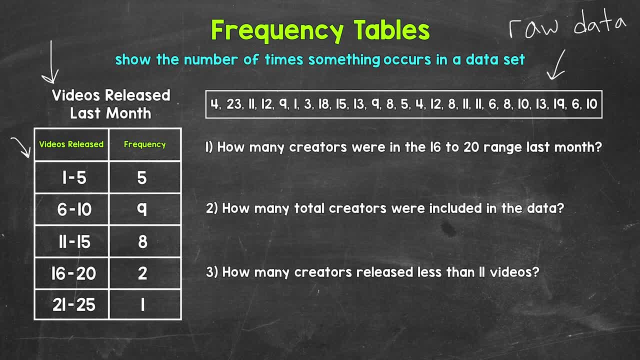 this is called grouped data, So these are the groups right here in the videos released column. If we have a wide range of data and a lot of individual values, using groups helps us create a more condensed and manageable table, Depending on the situation and the data. 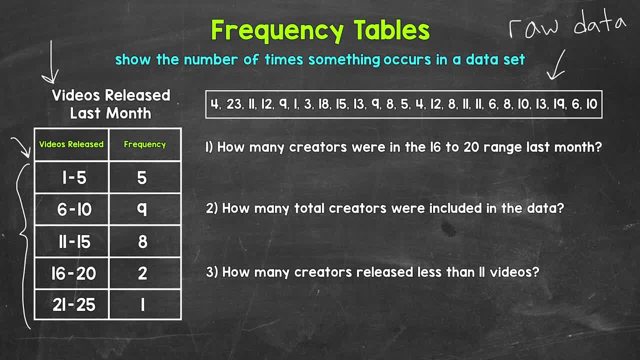 writing. each individual value could create a very long table. For example, for this data we would have to go from 1 to 23.. That table would be pretty long. So think about if we had an even wider table. If we had an even wider table, we would have to go from 1 to 23.. That table would be. a very long table. So if we had an even wider table, we would have to go from 1 to 23.. That table would be able to go from 1 to 23.. That table would be able to go from 1 to 23.. That table would be able to. 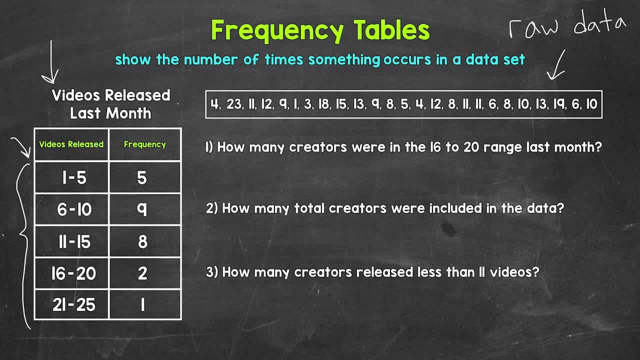 individual values, Maybe hundreds or even thousands of values. There are many ways to work with these groups, So these groups allow us to create a simpler and easier to work with table. Now, as far as the right column, So this column right here. this is the frequency, The number of times. 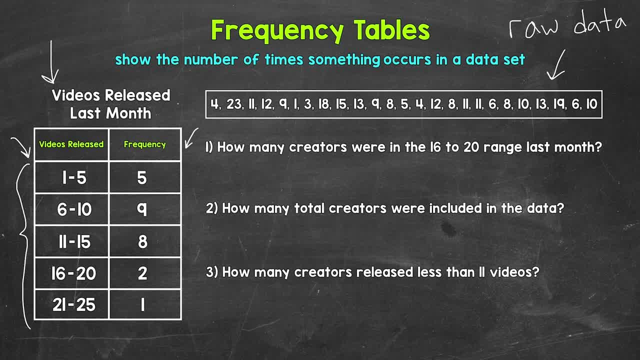 the values in our data show up within these groups. So, for example, taking a look and reading this, reading this table, how many creators released 1-2-5 videos last month? Well, 5 creators. How about 6-10 videos? Well, 9 creators. 11-15 videos: 8 creators. 16-20 videos: 2 creators. And then 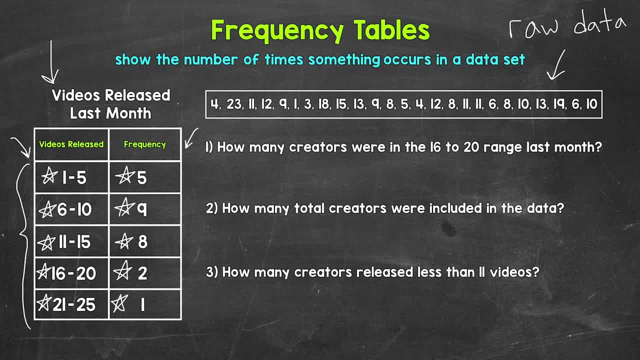 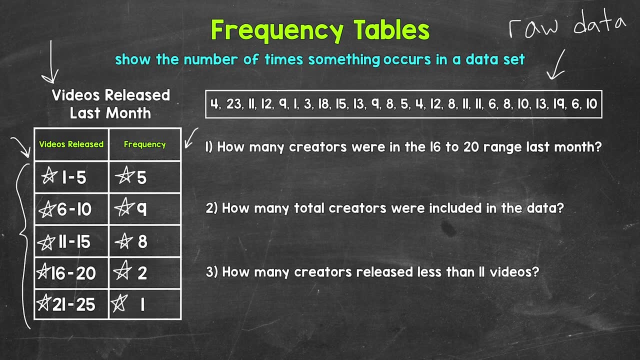 21-25 videos: 1 creator. So you can see that this frequency table really helps organize and present the data in a more meaningful and easier way to look at than just looking at the raw data. Now let's answer some questions regarding the data, Starting with number 1, where we have 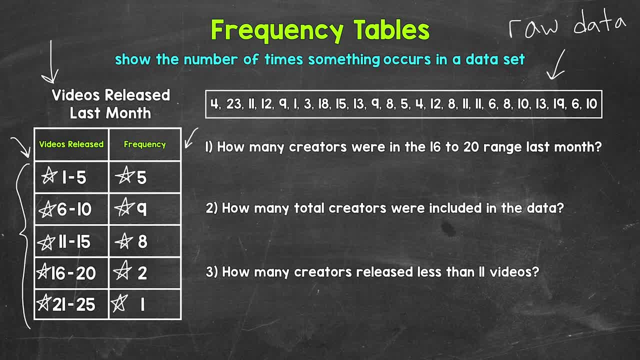 how many creators were in the 16-20 range as far as videos released last month. Here is 16-20 right here, So we have 2 creators. 2 creators released 16-20 videos last month, So they were in that range. Let's move on to number 2, where we have how many total creators were. 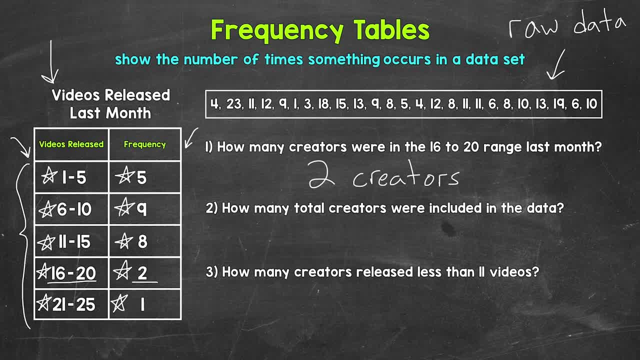 included in the data. Well, for this we need to take a look at the frequency column and add all of those numbers. So we have 5 creators, 9 creators, 8 creators, 2 creators and 1 creator. So if we add those up, 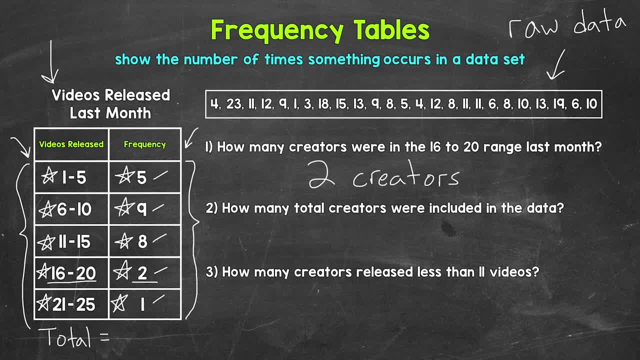 that's going to give us the total amount of creators. Well, 5 plus 9 is 14, plus 8 is 22,. plus 2 is 24, plus 1 gives us 25.. So 25 total creators. 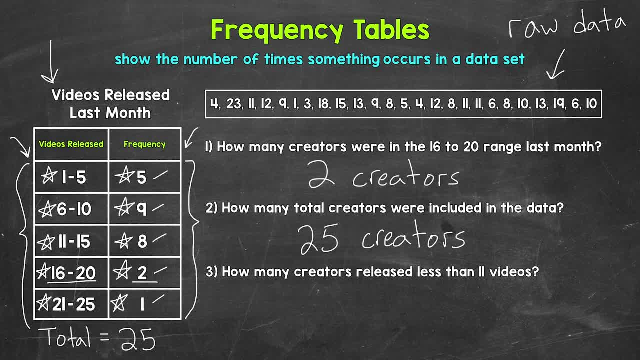 And then, lastly, let's move on to number 3, where we have how many creators released less than 11 videos. So less than 11, 11 is not included, So we are going to look right here. So the 6-10 and the 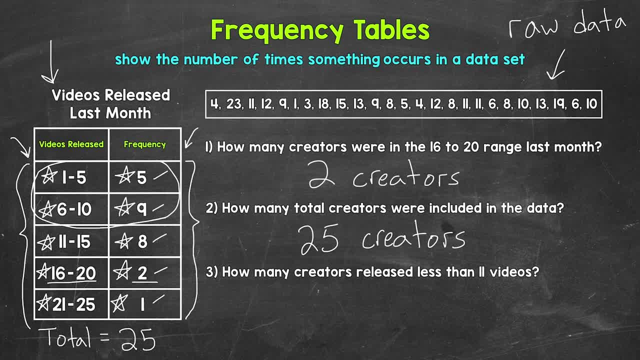 1-5 videos released. So we have 5 creators and 9 creators. So 5 plus 9 gives us the total amount of creators. So we have 5 creators and 9 creators. So 5 plus 9 gives us the. 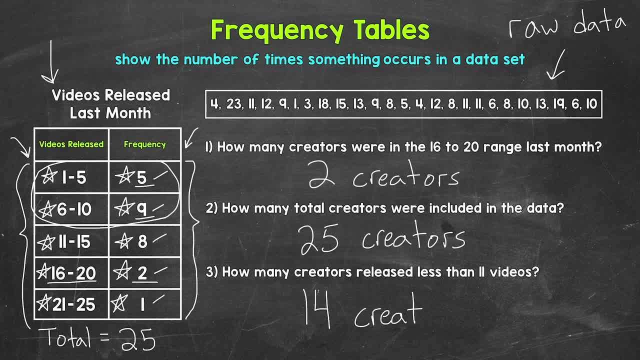 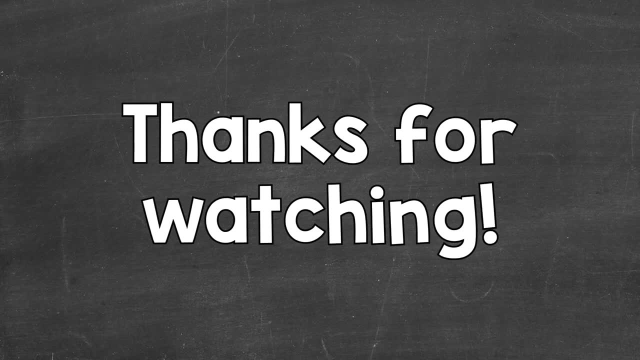 total amount of creators. So 5 plus 9 gives us 14 creators released less than 11 videos last month. So there you have it. There are the basics of reading and understanding ungrouped and grouped frequency tables. I hope that helped. Thanks so much for watching. Until next time, peace. Transcription by CastingWords.